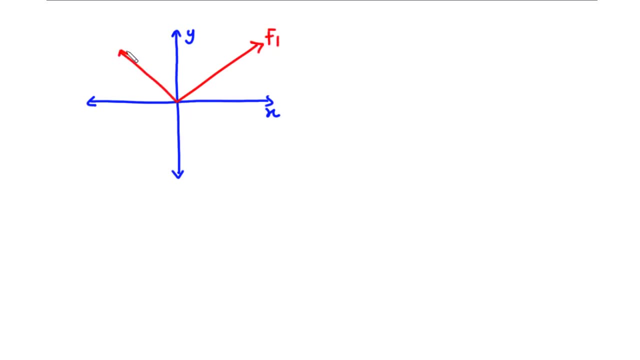 So we have this x-axis and this x-axis. Now let's assume that we have two forces acting in this plane. So we have this x-axis and this x-axis. Now each of this ancestor can be resolved into its i and j components. So, for example, i ii are being resolved to be f1, and then we have this to be f2.. 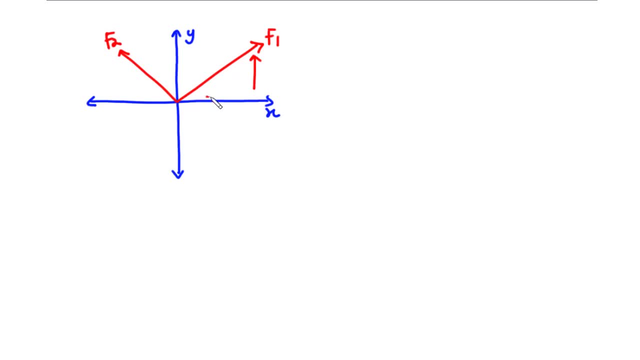 Now what we are saying is that each of these forces can be resolved into its i and j components. so for f1 we have f1, xi, and then f1, yj, and then also for f2 we have f2, xi, and then you have some forces caused by a support. 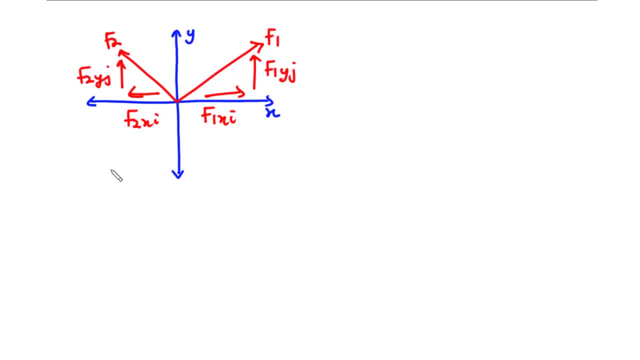 then F2Yj. So the two forces, F1 and F2, can be resolved into their i and j components. Now for equilibrium to be established, these forces must sum up to produce a zero. resultant force, that is, the summation of F, should be equal to zero. Now this can be expressed as: 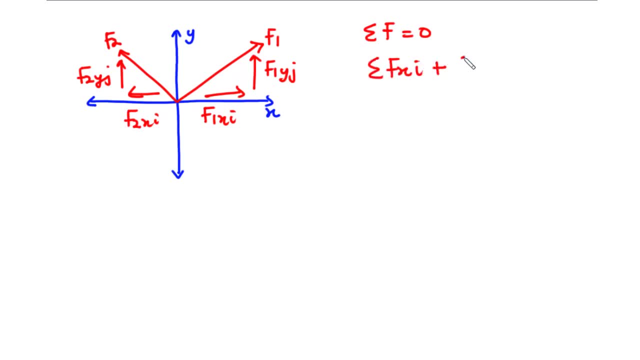 summation of Fxi plus summation of Fyj is equal to zero, And for this vector equation to be satisfied, the x and y component forces must all be equal to zero. That is, the summation of Fx should be equal to zero, as well as the summation of Fy must also be equal to zero. 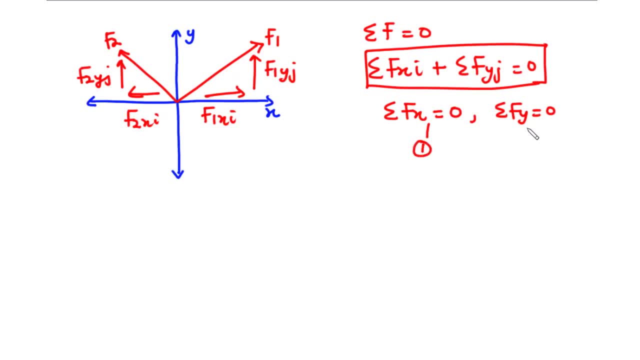 Now these two forces can be resolved into their i and j components. Now these two forces can be designed to utilize the union of two equations: summation of Fx equals zero, and then summation of Fy equals zero, produces at most two unknown's, which are generally. 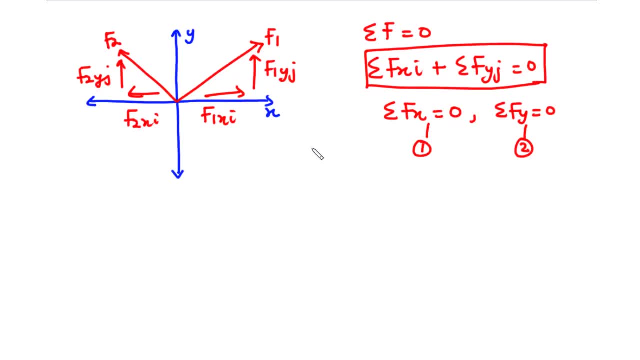 represented as angles and magnitude of forces shown on the particle's freebody diagram. Now, what, then, is a freebody diagram? a freebody diagram is a diagram that shows a particle and all the forces that act on this particular particle. So, given the two forces in this, 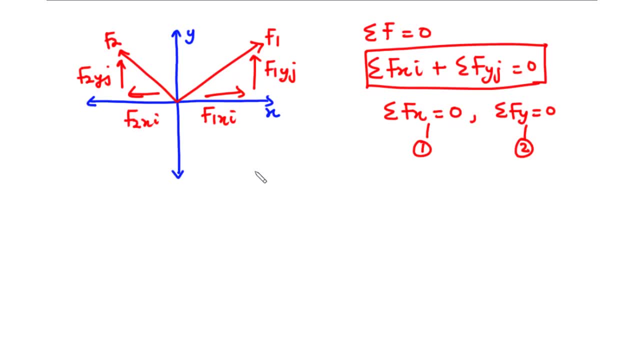 the best thing to do is to think of the particle as isolated and free from its surroundings, indicating all the forces that act on the particle. then you can move on to solve what the question demands from you. So, without wasting much time, let's take a few examples. 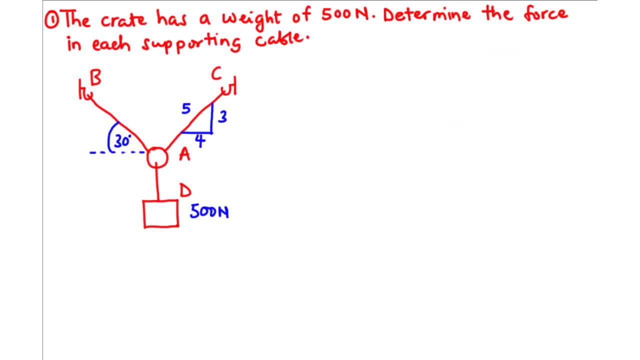 Now let's take the first example. The crate has a weight of 500 newtons. Determine the force in each supporting cable. So for this particular question we have three supporting cables: B, A, C, A and then A, D. 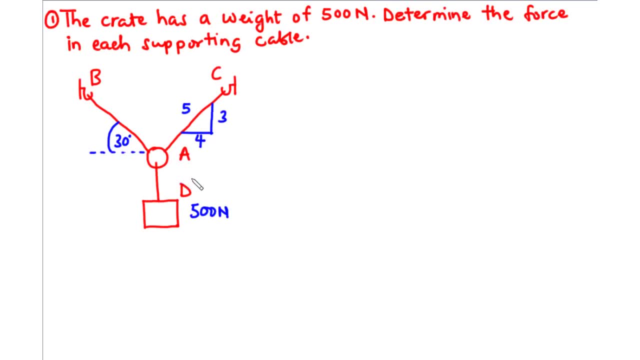 and all these three cables are linked together or connected together by a ring in the middle, And we have a crate attached at D. Now we are asked to find the forces in each of the supporting cables. So first of all, let's focus on the crate. 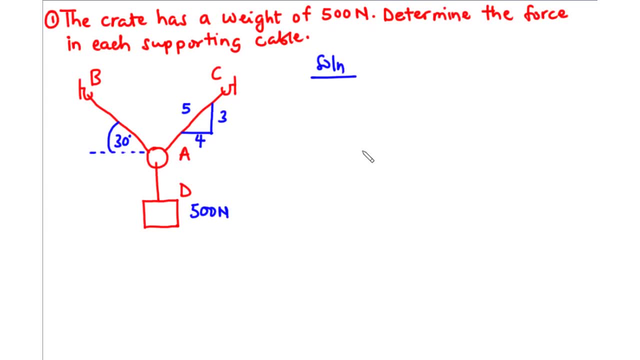 Now the crate is a support cable. The crate is said to have a weight of 500 newtons. So assuming we have this to be the crate, we have the weight of the crate acting vertically downwards. So that is, W equals 500 newtons. 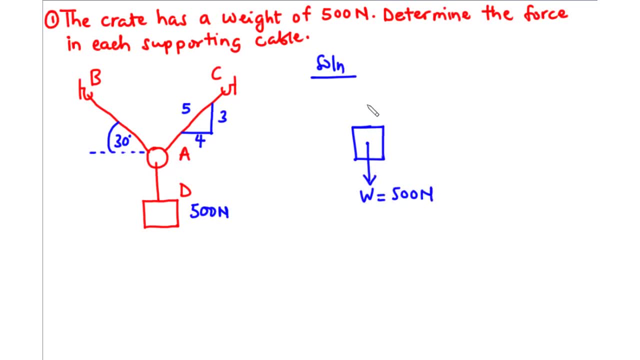 Now this weight is going to exert an upward tensional force in the cable, That is, the cable TAD, which is equal to the magnitude of the force. So this is the magnitude of the weight, except that it acts upward, So that even though the two forces have the same magnitude, 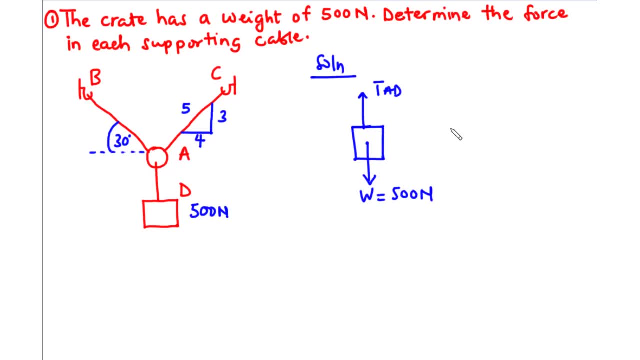 they act along different directions. So let's assume that the weight force acting vertically downwards has a negative value. So we have negative W, plus the tensional force which acts upwards has a positive value, That is TAD, And we say that this is equal to zero. 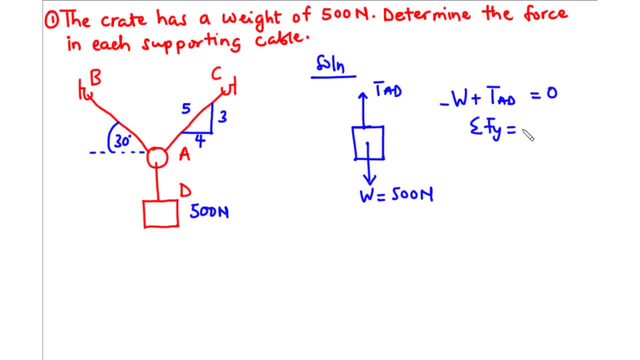 Therefore, the sum of forces along the y-axis is equal to zero. Hence we say that equilibrium has been established. So at this point, let's investigate the equilibrium of the ring at A, And we are going to do that by drawing a free body diagram. 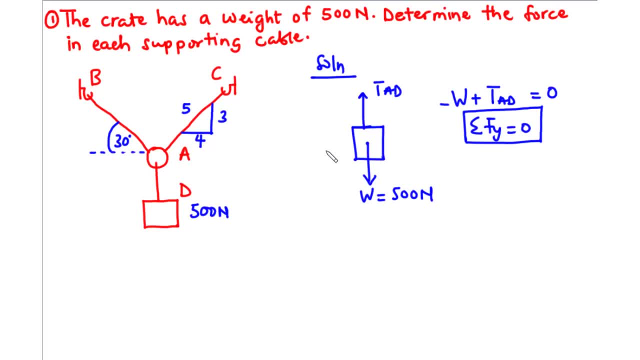 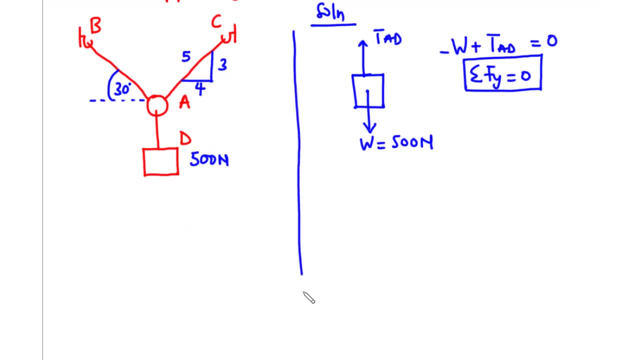 indicating all the forces that act on the crate. And we are going to do that on the XY plane. So let's draw the XY plane. So we have this to be the y-axis, We have the x-axis. Now let's indicate all the forces acting on the crate. 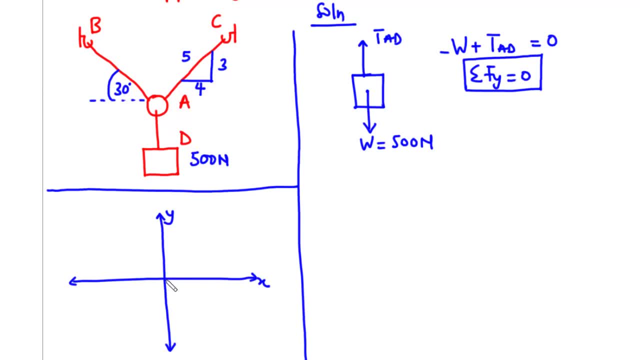 So we have the weight of the crate acting vertically downwards. We have W equals 500 Newtons, that is the weight of the crate, And the upward tensional force it exerts in the cable TAD is distributed between the two cables, TC and then TB. 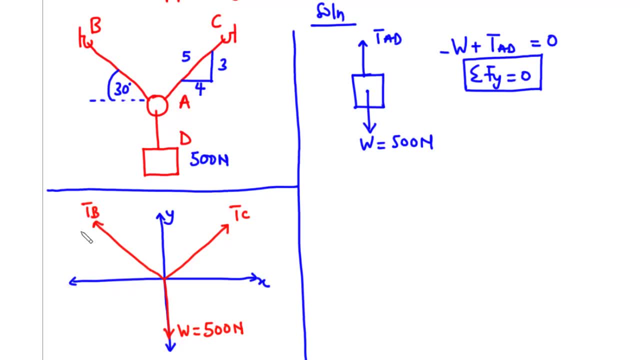 Now we have the angle between the negative x-axis and then TB to be 30 degrees, And then here we are provided with a small slope triangle, that is a 3-4-5 triangle. So basically, what we are going to do is to calculate the tensional force in TC and also 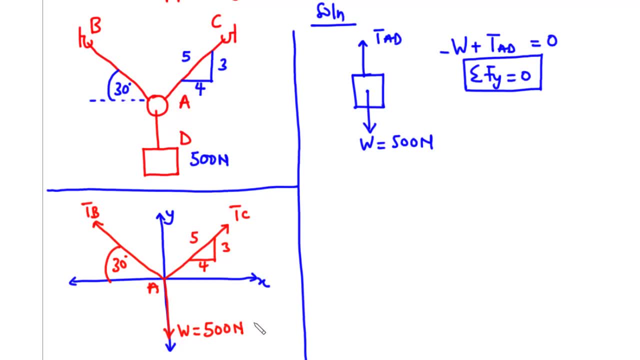 in TB. So, basically, what we are going to do is to calculate the tensional force in TC and also in TB, So applying the equations of equilibrium along the x and y-axis. Now let's start off with the x-axis. Now we said that the summation of Fx should be equal to zero. 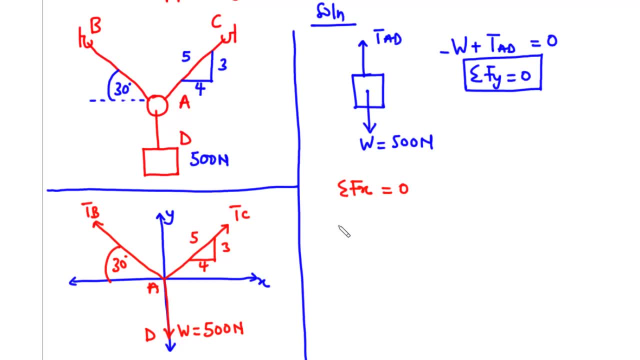 Therefore, let's find the sum of component forces acting along the x-axis. So how do we apply the small slope triangle? Now we know that the x component of TC acts along the x-axis. Now we have four corresponding to the value on the x-axis. 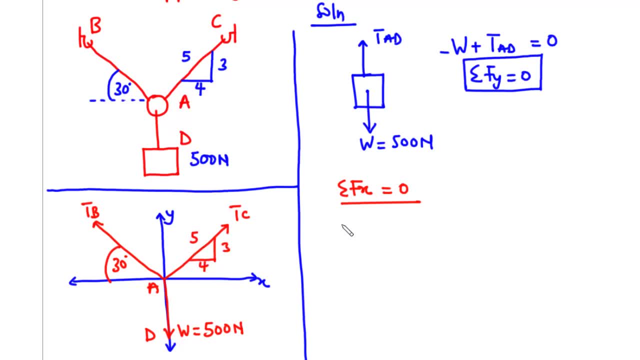 And we know that cos theta is equal to adjacent over hypotenuse, Therefore we say that TCx is equal to 4.. So that is the adjacent divided by the hypotenuse, that is Tc, And then Tc also corresponds to 5.. 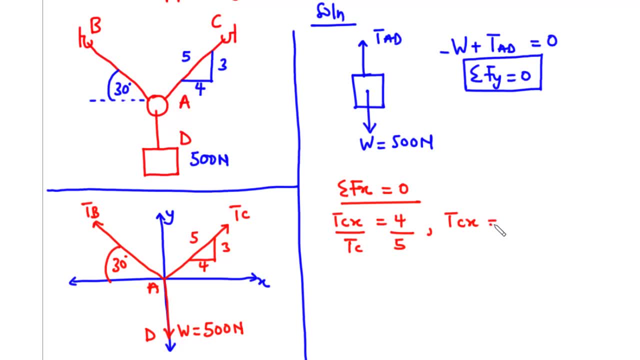 Therefore we say that Tcx is equal to 4.. Let's start defending. And to the left of the table is the thickness and the line is set as a K. Let's see: canво check is equal to 4 over 5 times tc. So this is the value of tcx. Notice that tcx acts along. 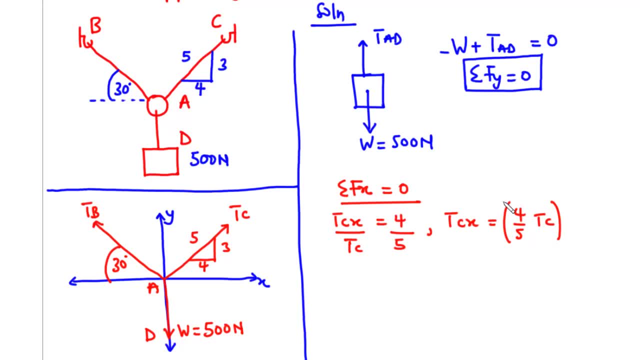 the positive x-axis. Therefore, we still maintain this value as positive. So for tbx, we have tbx acting along the negative x-axis, So this is tbx. And then we have tby acting along the positive y-axis. So for tc, we have this also to be tcx and then this to be tcy. Now 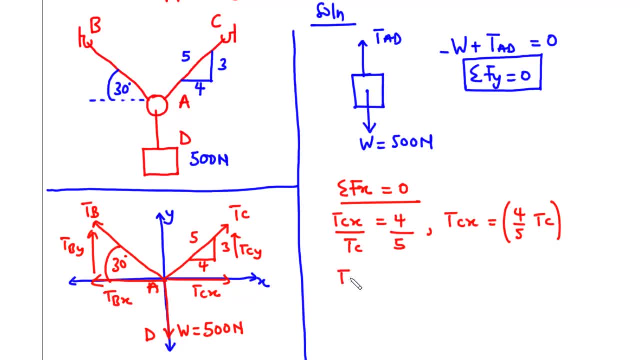 let's continue So to find tbx. tbx is simply tb cos 30.. Notice that since tbx is acting along the negative x-axis, we need to negate this value. Therefore, tbx is equal to negative tb cos 30.. So now let's 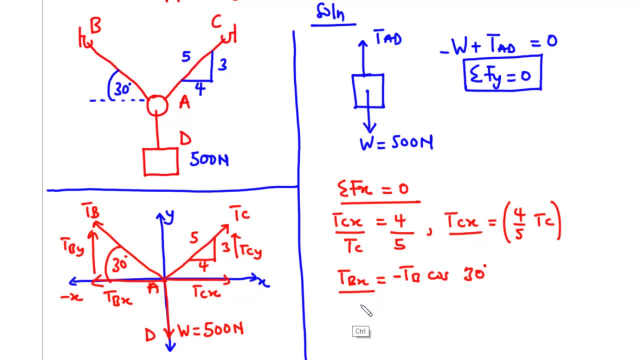 add the two values tcx and then tbx, and then equate to zero according to the equilibrium equation. So we have tcx plus tbx equals zero. tcx can be simplified as: 0.8 tc plus negative tb. cos 30 equals zero. Therefore we have 0.8 tc and then cos 30 gives 0.8660.. 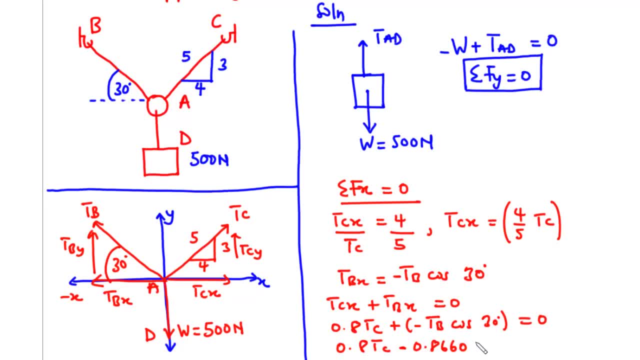 So we have negative. 0.8660 tb equals zero. Now let's make tc the subject. So we have tc equals. This is to the right hand side, So that becomes 0.8660 tb, and then we divide through by 0.8.. 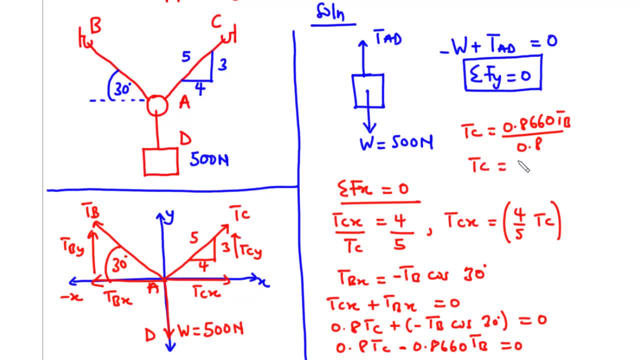 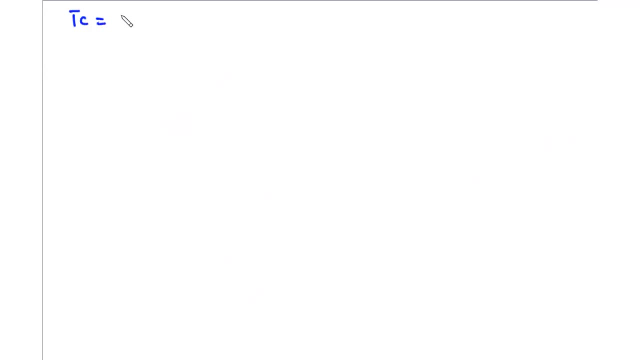 Therefore, we have tc to be equal to 1.0825 tb. Now let's call this equation 1.. So for equation 1. We had tc equals 1.0825 tb. tc equals 1.0825 tb. 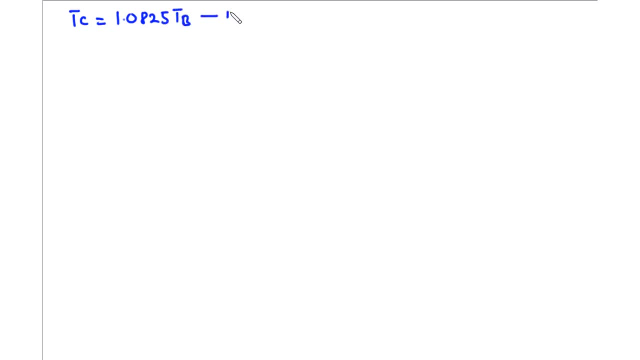 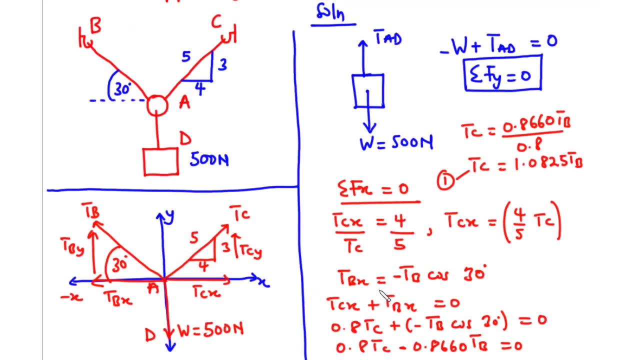 tc equals 1.0825 tb. Now let's consider the forces along the y-axis. So for the forces along the y-axis, we have Tcy, we have Tby and then W, which is the weight of the crate. So for Tcy, we have Tcy acting along the positive y-axis and that corresponds to 3.. 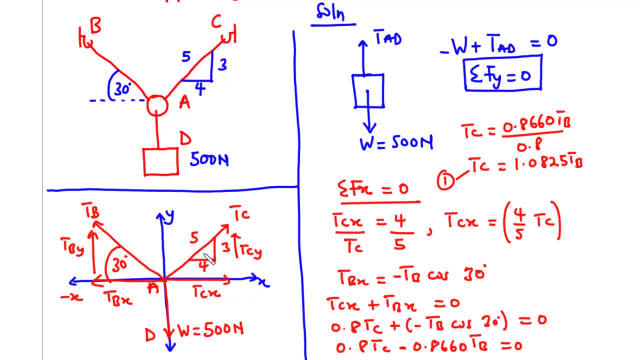 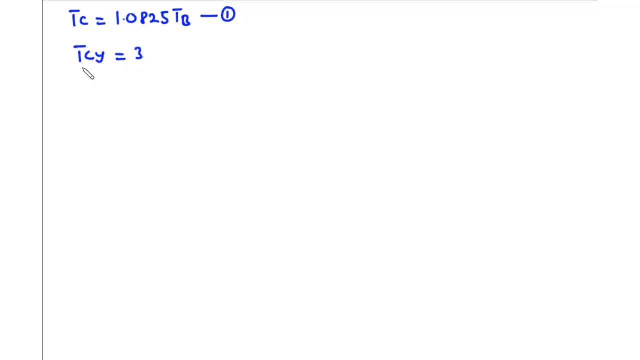 So since sin theta is equal to opposite over the hypotenuse, then that is basically 3 over 5.. So we have Tcy equals 3 divided by Tc equals 5.. So this becomes: Tcy equals 3 divided by Tc equals 5.. 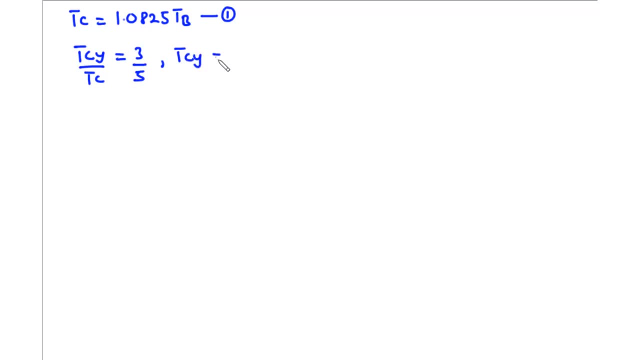 So, by the way, we have Tcy acting along the positive y-axis And by this we can say that Tcy is equal to 3 over 5 Tc, And 3 over 5 is the same as 0.6.. 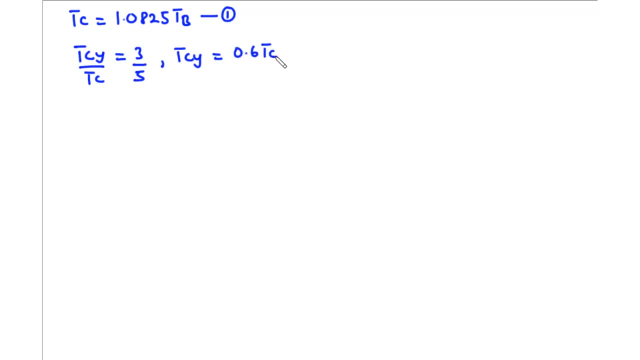 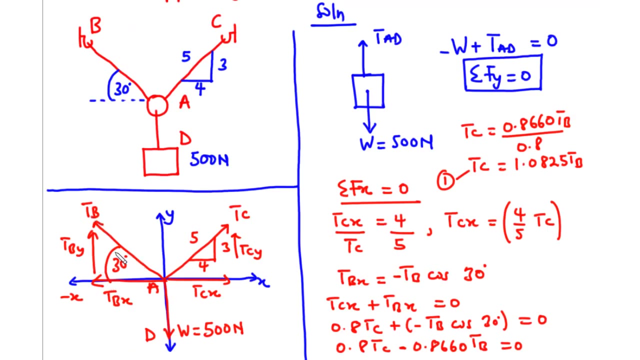 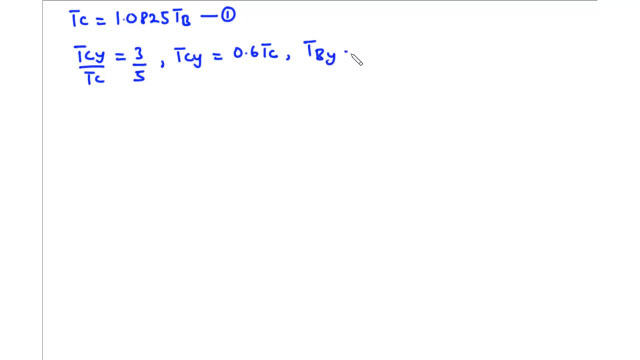 So we can basically write 0.6 Tc And for Tby, Tby is simply Tb sin 30.. So we have Tby equals 3 over 5 Tc. So we have Tby equals 3 over 5 Tc. 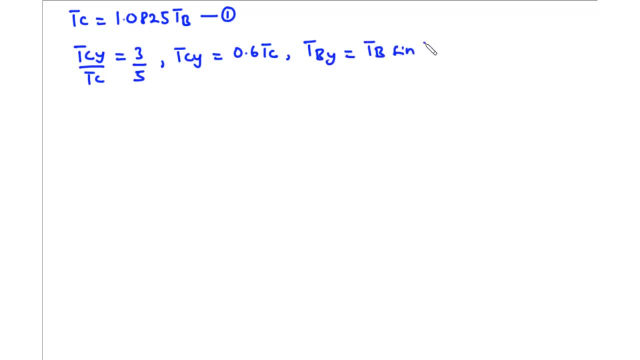 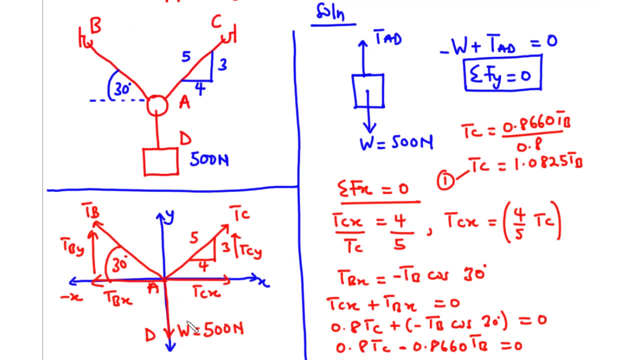 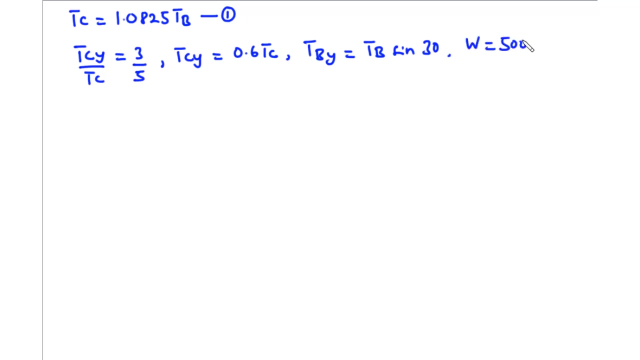 So we have Tb sin 30.. Tb sine 30.. Notice that all these two component forces are acting along the positive y-axis. and then we have the weight force acting along the negative y-axis. So it means that we are going to negate this value. So we have: W equals 500 newtons. Good, So we know that. the summation of 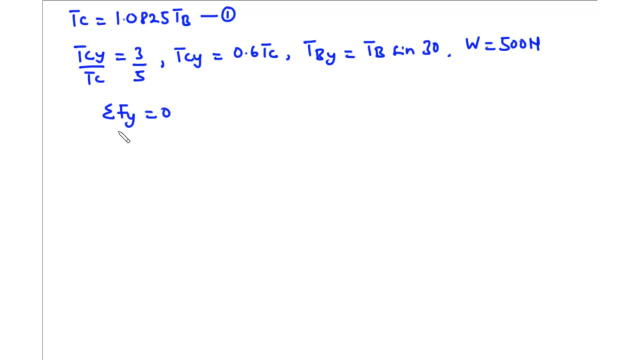 the forces along the y-axis should be equal to zero. Therefore we have Tcy plus Tby. minus W equals zero, Negative because it's acting along the negative y-axis, It's acting vertically downwards. So now let's put in the values of Tcy, Tby and then W, So for Tcy we have 0.6 Tc. 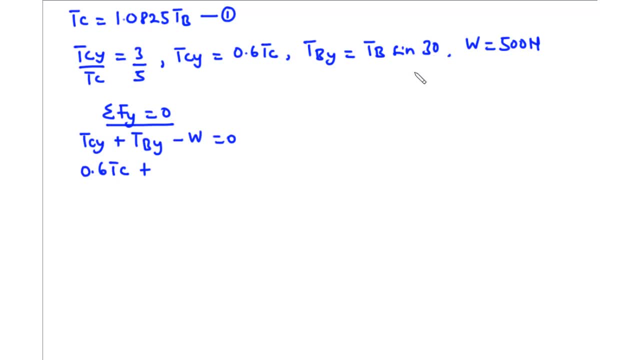 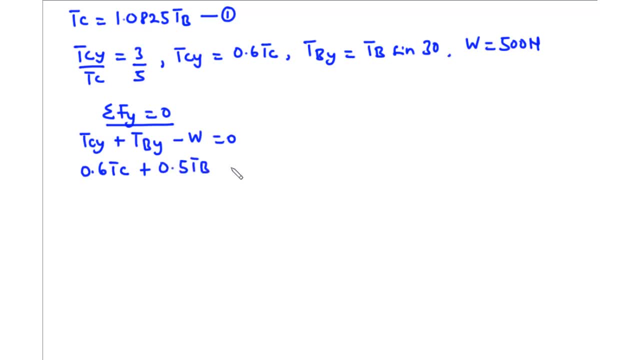 0.5 Tb minus 500 equals zero. Now we are going to transpose negative 500 to the right hand side. Therefore, we have 0.6 Tc plus 0.5 Tb equals 500.. Now let's call this equation two. Don't forget that we had equation one to be. Tc equals 1.0825 Tb. 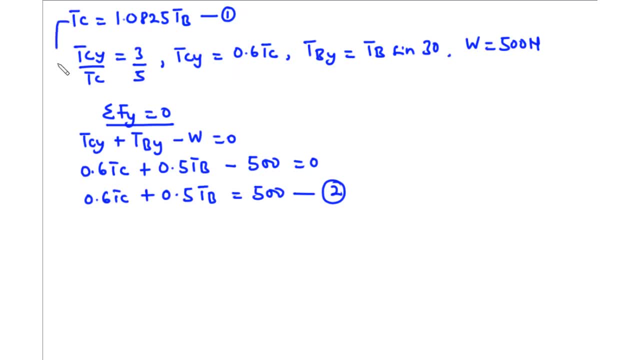 So we are going to substitute this value into equation two. So let's do that, So this becomes 0.6.. We have Tc to be 1.0825 Tb, And then plus 0.5 Tb equals 500.. 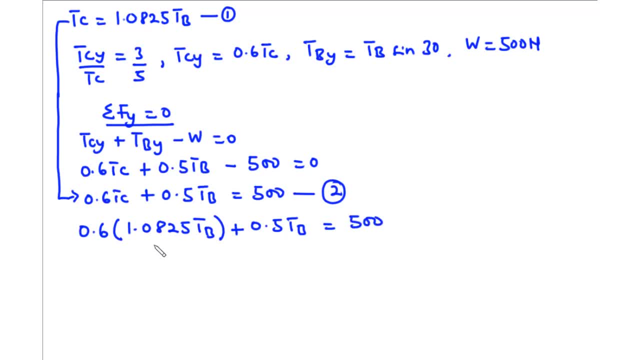 So 0.6 times 1.0825 gives 0.6495 times Tb. plus 0.5 Tb equals 500.. So when you add these two values you get 0.6 times 1.0825, Tb equals 500.. 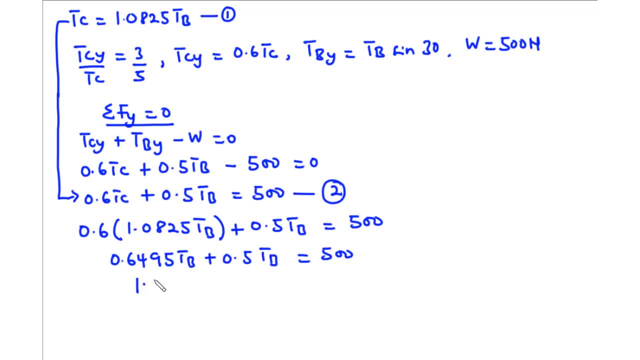 So when you add these two values, you get: 0.6 times 1.0825: Tb equals 500.. So when you add these two values, you get 0.6 times 1.0825, Tb equals 500.. You divide through by 1.1495: 1.1495.. 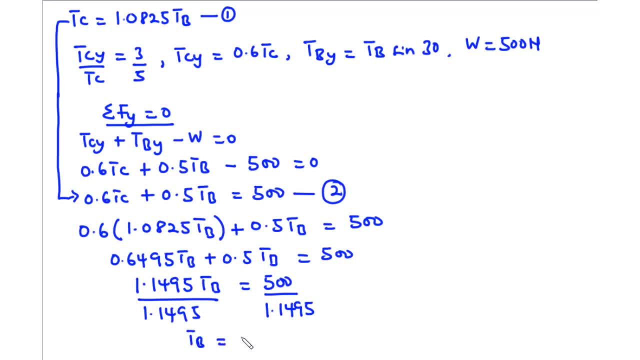 So that we have Tb to be equal to 434.97 Newton's, So that we have Tb to be equal to 434.97 Newton's. Therefore, we can round on the left. So Crunch っ. these two values work together. 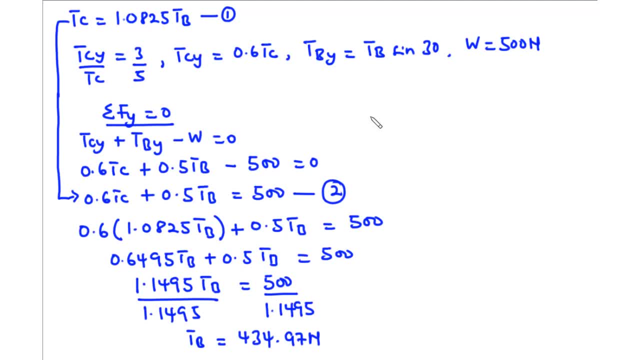 But we can round this one up to the nearest whole number, as Tb equals 435N. So this is the value of Tb, the tension in the cable, Ba. Now let's solve for Tc, So we have Tc also to be equal to 1.0825.. 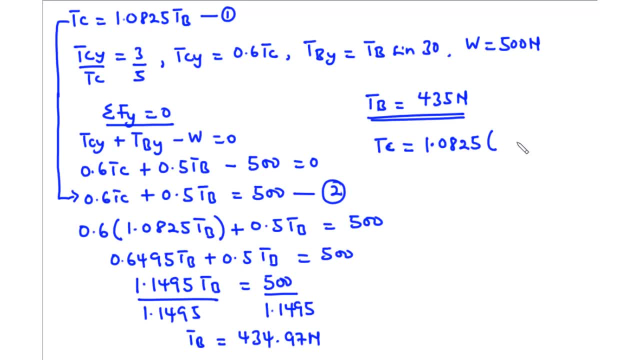 Now we are going to multiply this by Tb, So we have 434.97.. So after multiplying the two values, we are going to get 470.85.. Rounding this up to the nearest whole number, we have 471N. 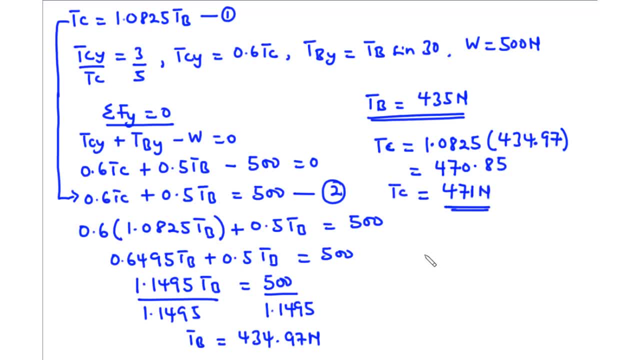 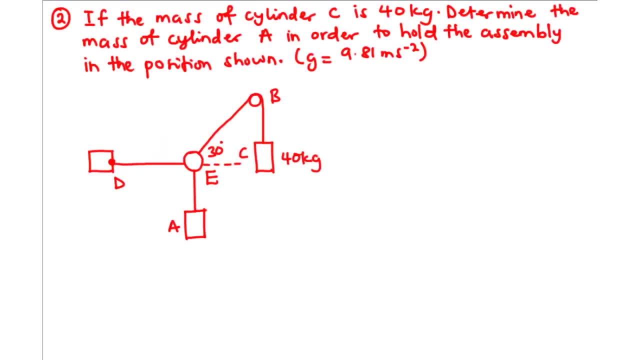 This is the value of Tc, the tension in the cable, Ca. Now let's move on as we take the next example, So to example 2, if the mass of cylinder C is 40 kg, determine the mass of cylinder A in order to hold up the assembly in the position shown, given that acceleration due 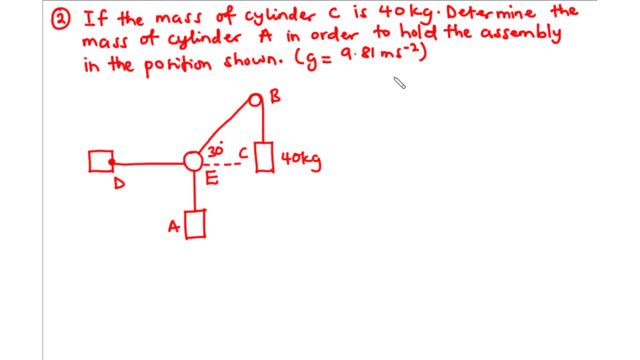 to gravity is equal to 9.81 m per second square. Now for this diagram. we have three cables. We have the cable De E A And then the cable that extends from E through to B to C. Now we are not given the weight of cylinder A. However, we are asked to find the mass. 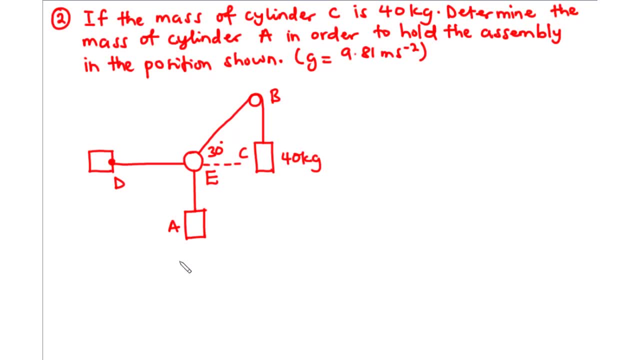 of cylinder A. Now we know that weight is given by mass times- acceleration due to gravity. Therefore, the weight of A is equal to the mass of A times G. Now we have G to be 9.81, therefore we have the weight to be 9.81 times ma. 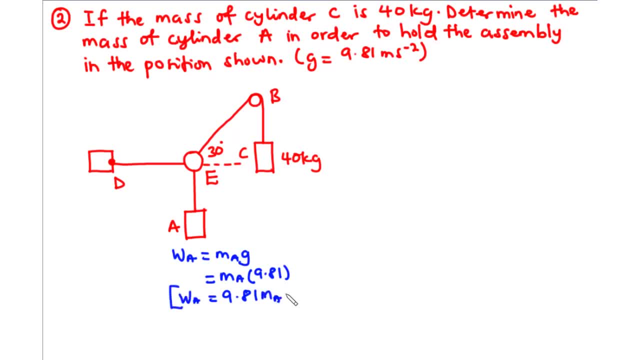 So that is the weight of cylinder A. Now let's focus on the two cylinders Now, since we want to find the mass of cylinder A, then we need to focus on the sum of forces along the y-axis, Because we have no business calculating for sum of forces along the x-axis, so we just 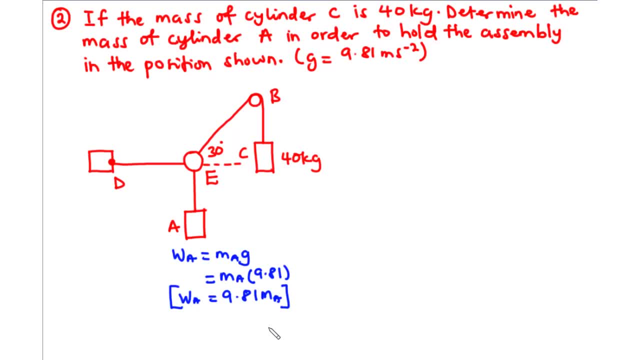 need to focus on the sum of forces along the y-axis. Now, considering cylinder A, We are going to have the weight of this cylinder acting vertically downwards, So that is wa equals 9.81 times ma. This tells us where of разные magnitudes act. the looms are called vr. 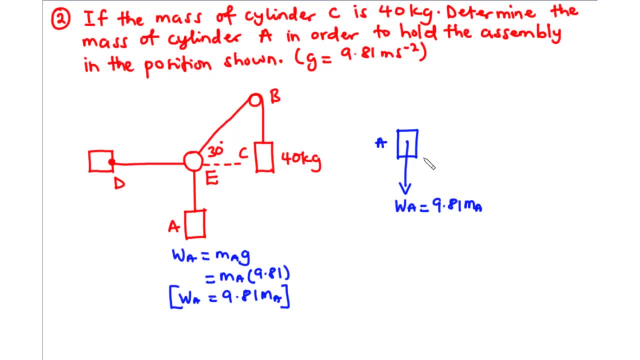 Now that becomes w million. 3.3% was the mass according to Mor整 x, And this weight is going to exert an upward tensional force in the cable EA. So that is going to be TEA. Notice that they have the same magnitude. however, they act along opposite directions. 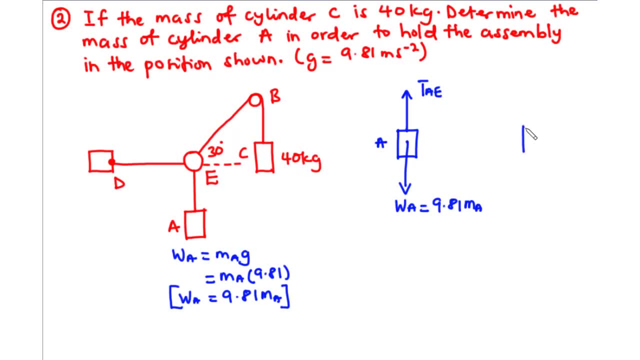 Now let's focus on cylinder C. Now for cylinder C we have the mass to be 40 kilograms. So the weight of cylinder C becomes 40 times 9.81, and that is equal to 392.4 Newtons. So this is the weight of cylinder C. Now, at B there is a pulley. 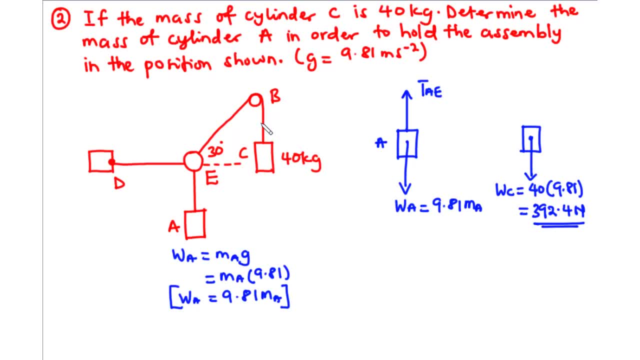 Now the weight of cylinder C pulls this rope downwards, which exerts a tensional force equal to the magnitude of the weight of cylinder C In this cable. And this makes a lot of sense because we have the same cable across the pulley. Therefore, if the weight of cylinder C pulls this cable downwards, then it's going to exert 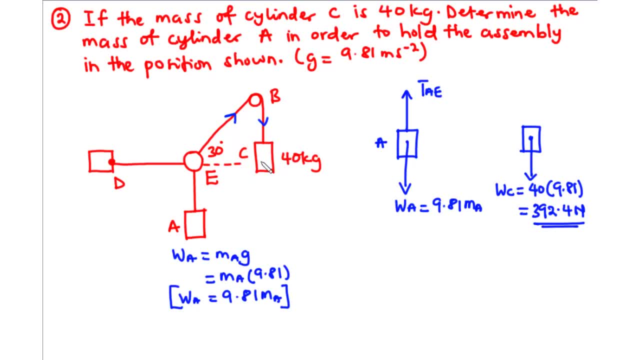 a tensional force of the same magnitude as the weight of cylinder C in this cable. Therefore we say that the tension in the cable at B is equal to 392.4 Newtons. Thus TB is equal to the weight of cylinder C. Now let's represent this on the XY plane. 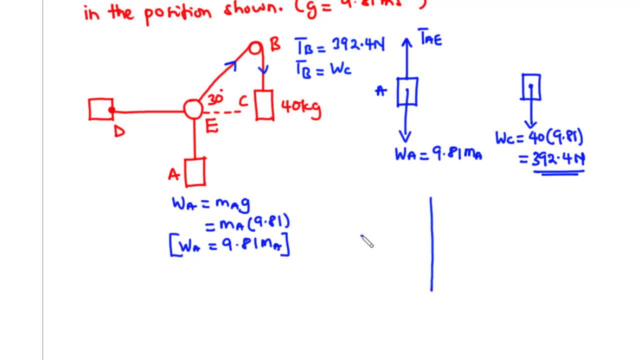 So on the XY plane, we have the Y axis, we have the X axis, we have WA to be the weight of cylinder A. So this is WA, the weight of cylinder A, 9.81 times MA. Now we are going to ignore the weight of cylinder C, because it is the same as the magnitude of 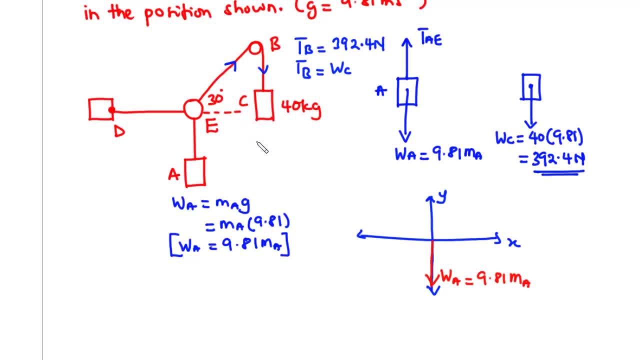 the tension in the cable at B. So we are going to ignore the weight of cylinder C as we introduce the tension in cable B. So this is WA. The weight of cylinder C is equal to 392.4 Newtons. Thus TB is equal to 392.4 Newtons. 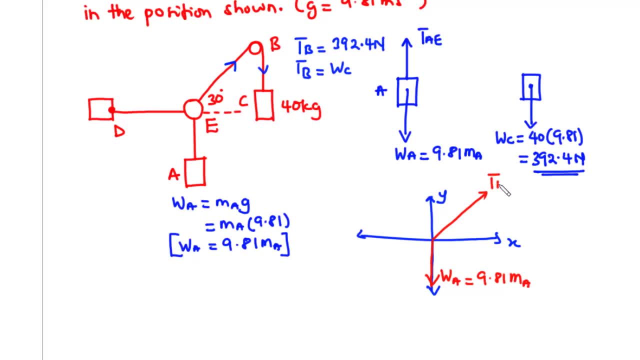 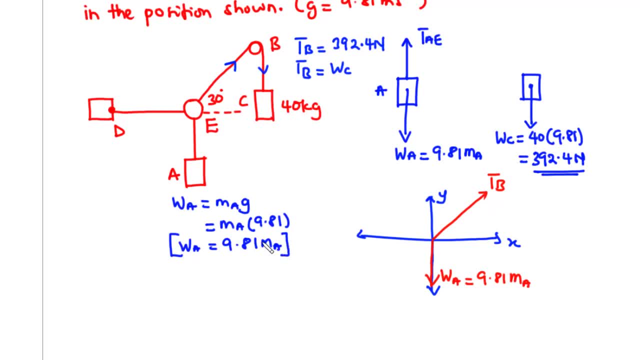 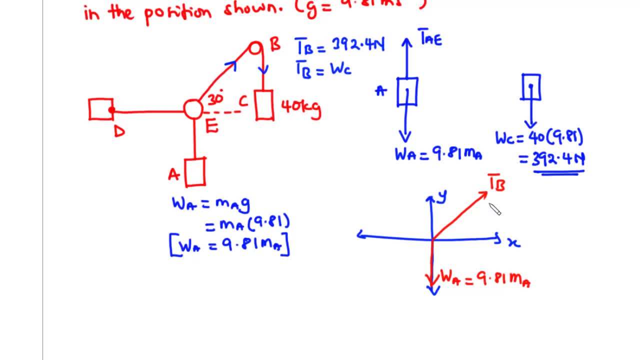 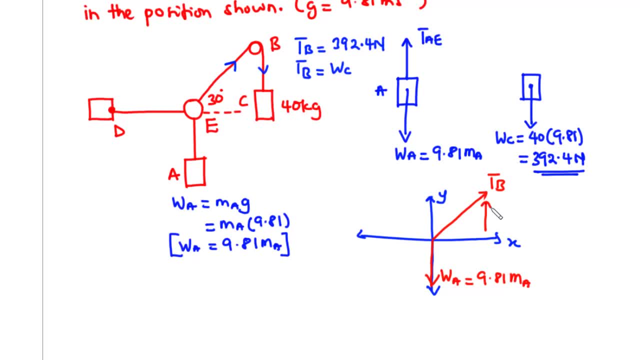 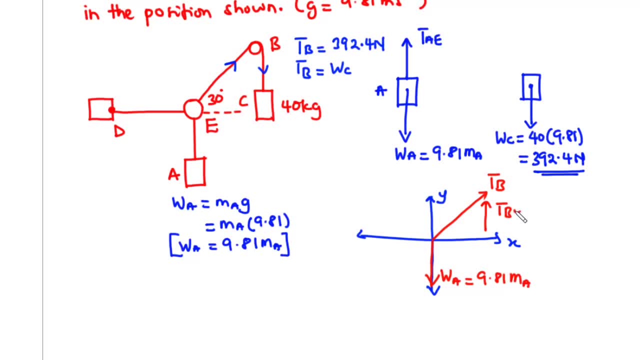 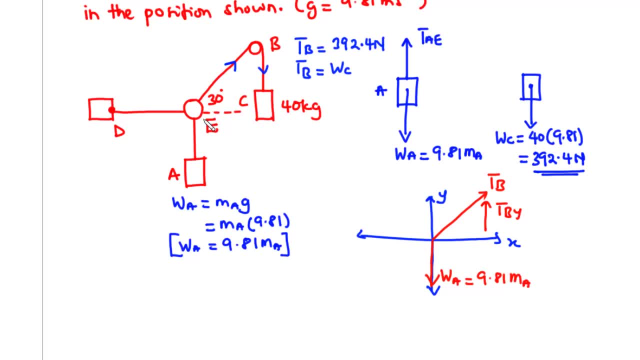 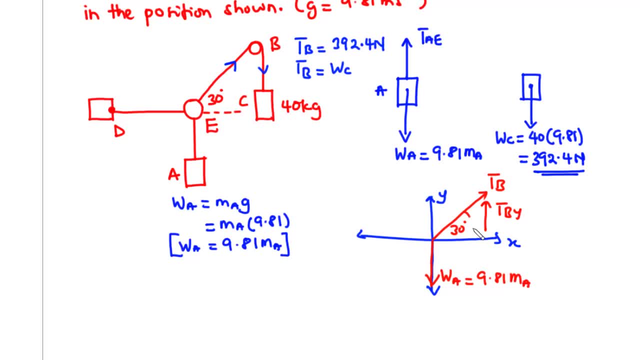 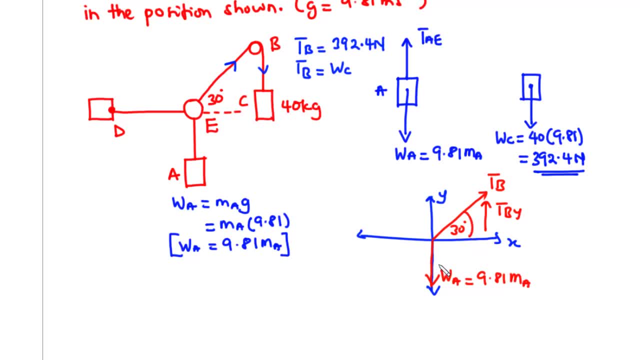 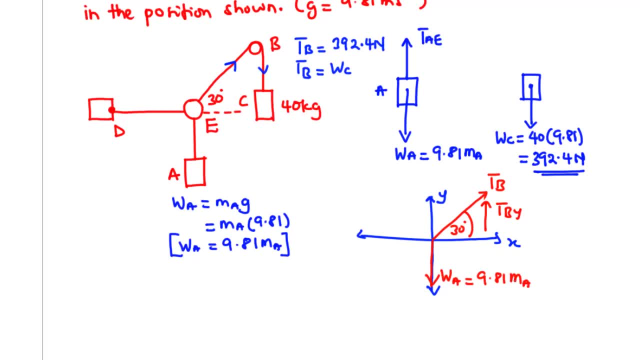 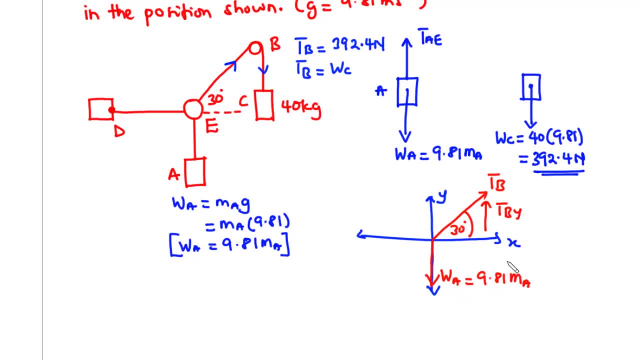 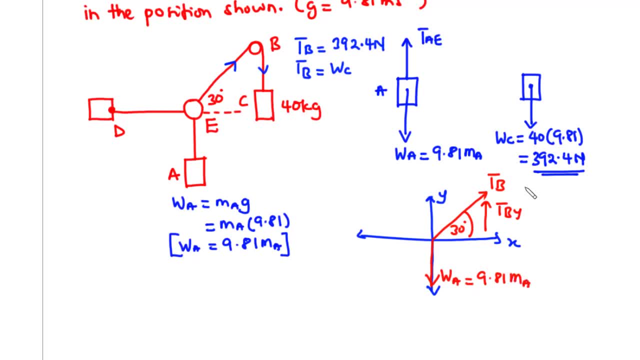 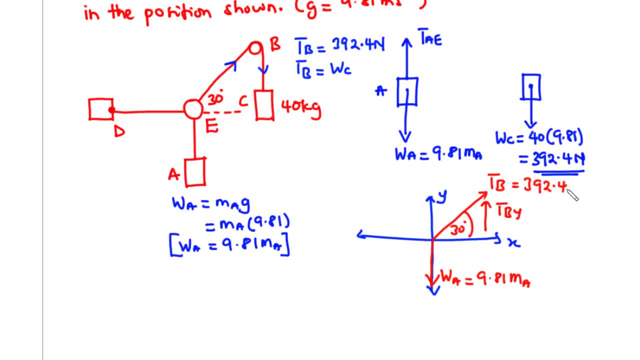 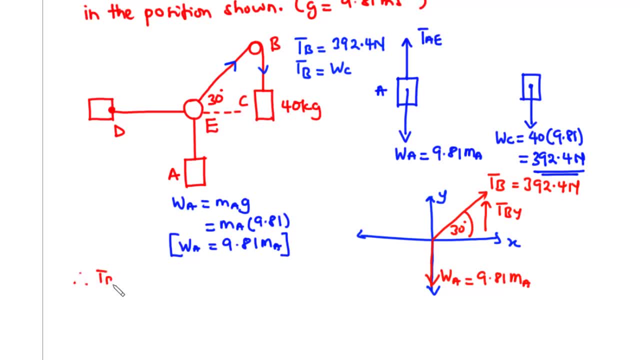 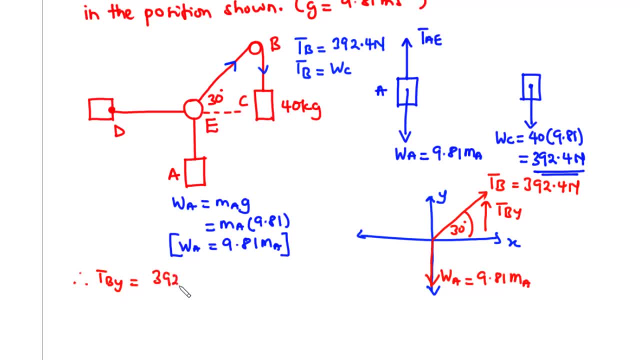 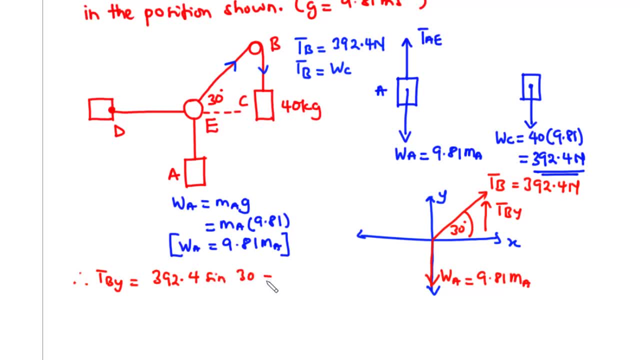 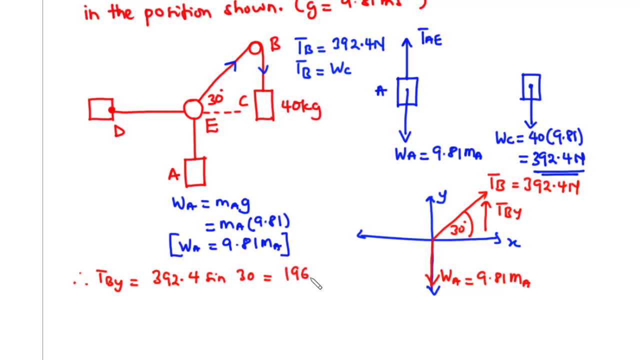 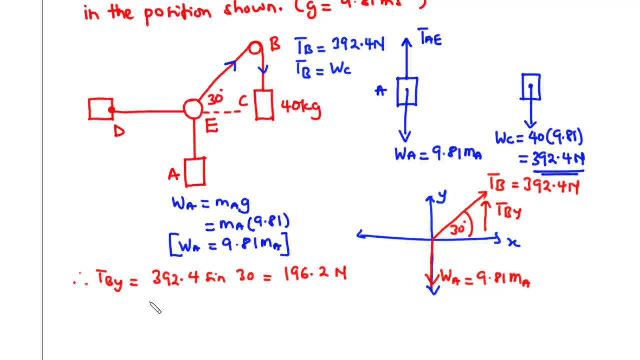 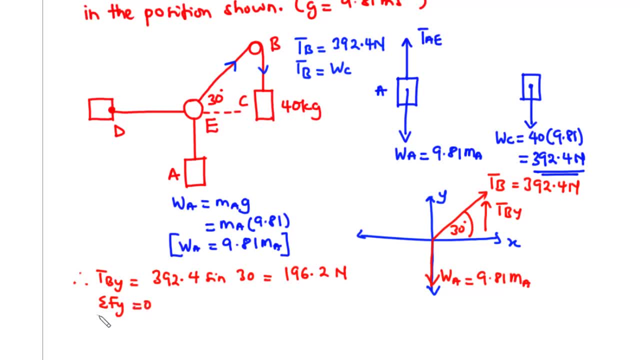 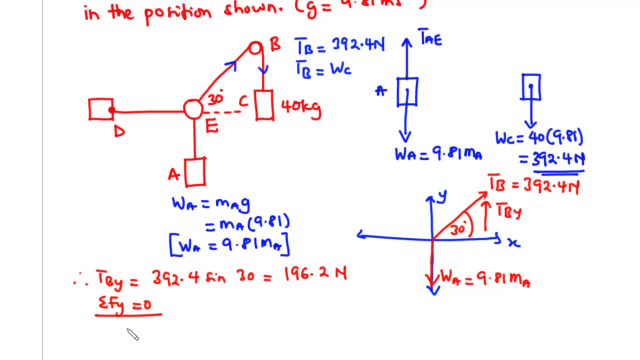 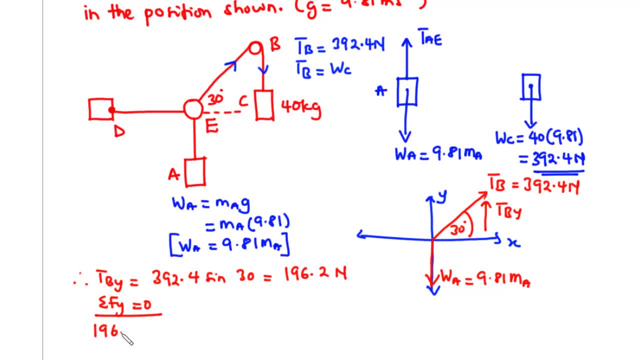 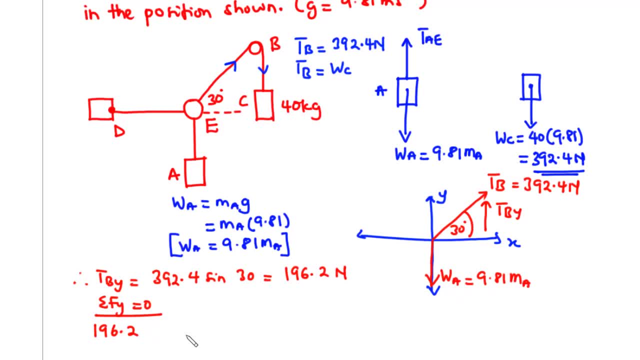 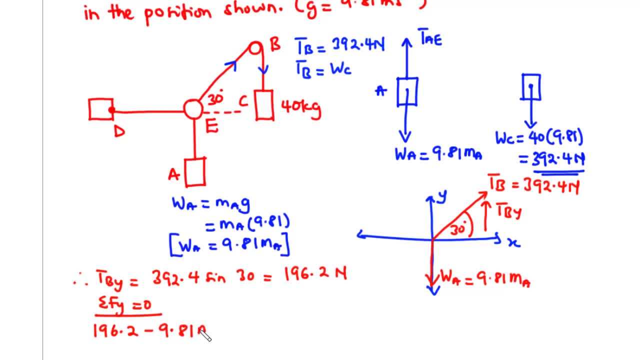 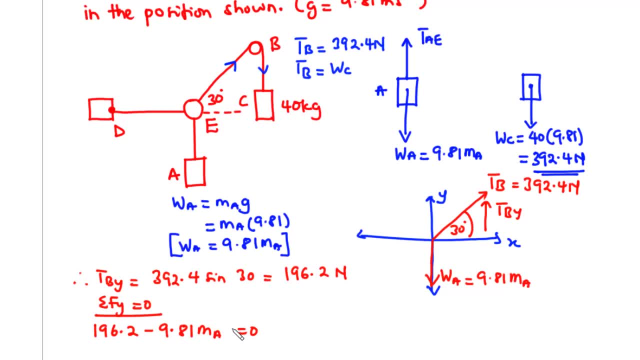 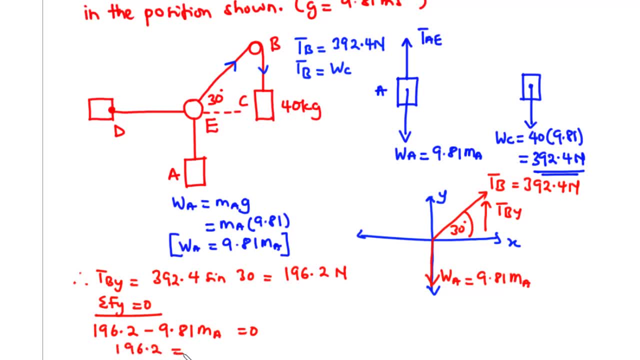 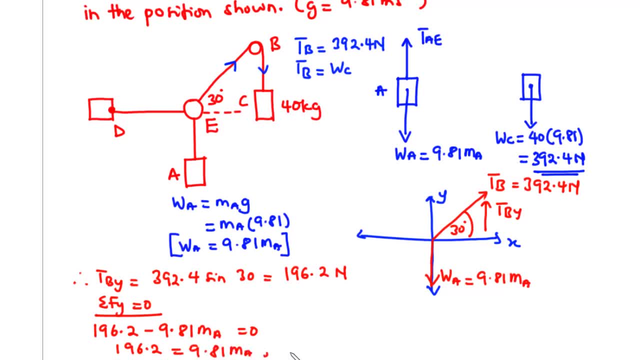 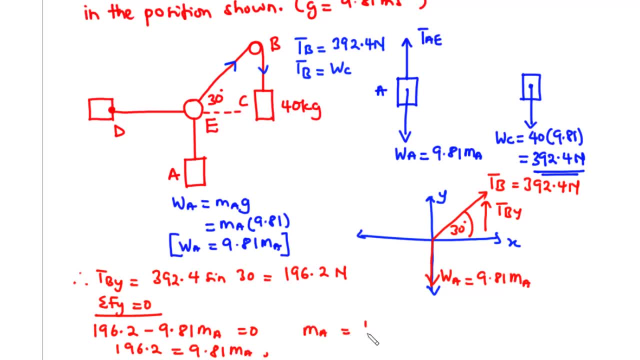 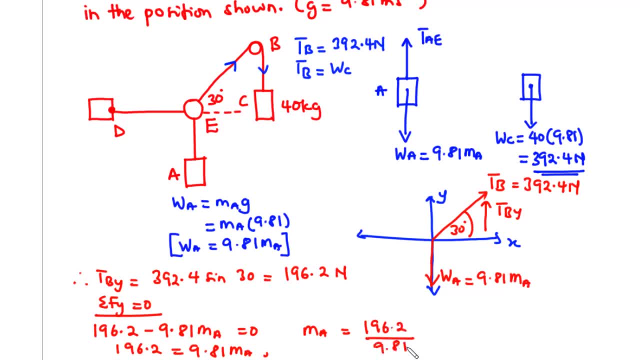 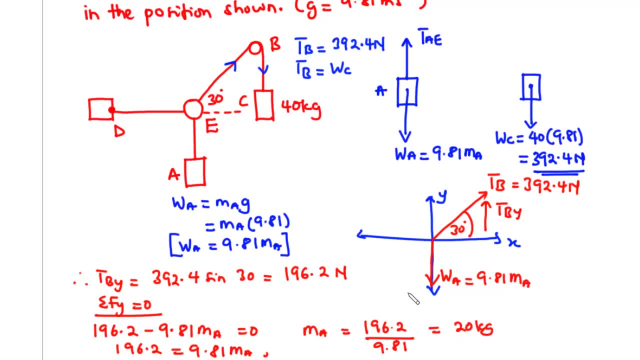